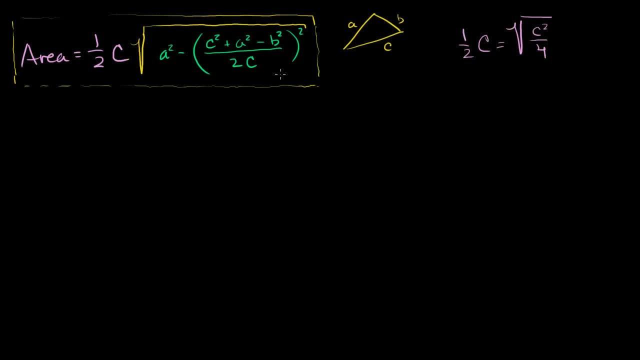 squared over 4.. You take the square root of that, you get 1 half c. So this whole expression is equal to: instead of drawing the radical, I'll just write the square root of this of c squared over 4, times all of this. 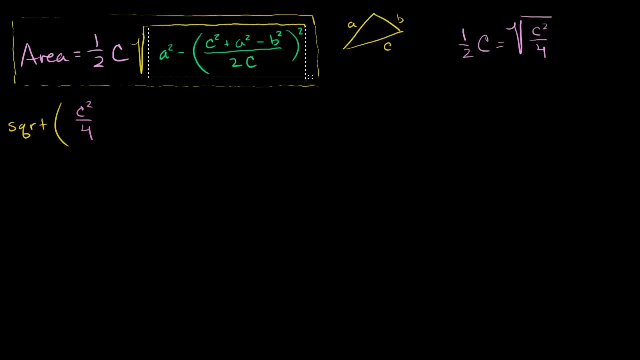 Times. I'll just copy and paste it. times all of that. Copy and paste, So times all of that, And of course it has to be distributed. So c squared over 4 times all of that, And then we have to close the square root. 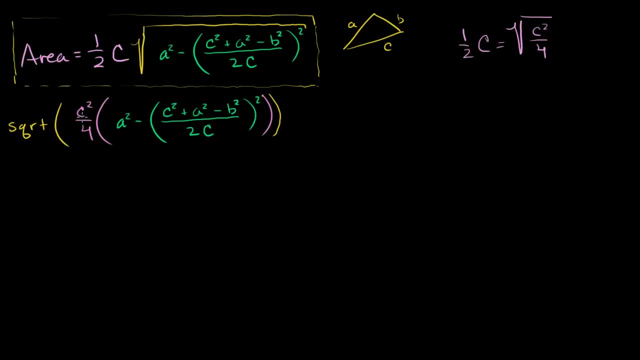 And then this thing: let me just distribute the c squared over 4, this is going to be equal to the square root. This is going to be hairy, but I think you'll find it satisfying to see how this could turn into something as. 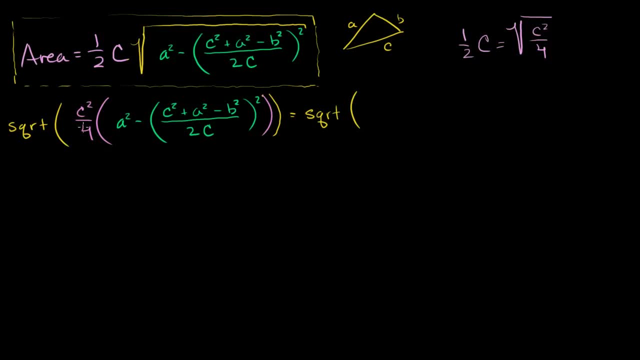 simple as Heron's formula. The square root of c squared over 4 times a squared is c squared a squared over 4.. Minus c squared over 4.. c squared over 4,. I'm just distributing this Times and I'm going to write it as the numerator squared. 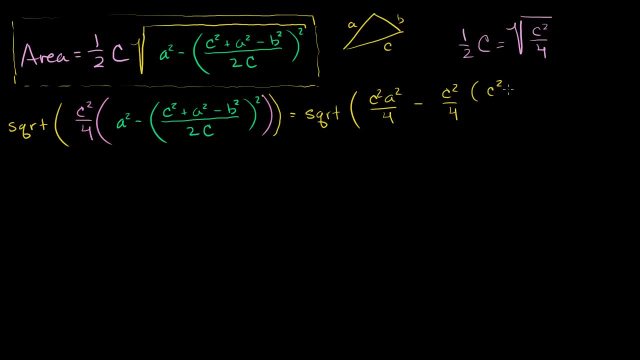 over the denominator squared. So times c squared plus a squared, minus b squared, squared over. if I square the denominator, that's 4c squared And we immediately see that c squared and that c squared are going to cancel out. Let me close all of the parentheses. 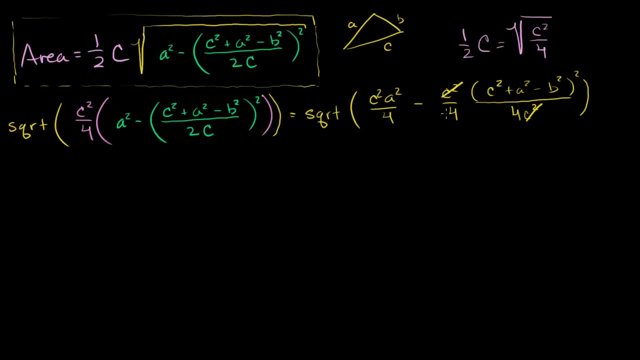 Just like that. And then, of course, this 4 times that 4, that's going to result in- let me write it this way: That's the same thing as 4 squared, Instead of writing 16,. you'll see why I'm writing that. 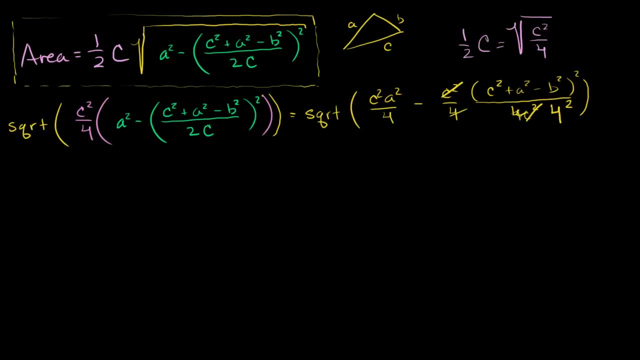 Now this I can rewrite. as this is going to be equal to the square root, I'm arbitrarily switching colors of c a over 2 squared. This is the same thing as that, right? I'm just writing it as the whole thing. 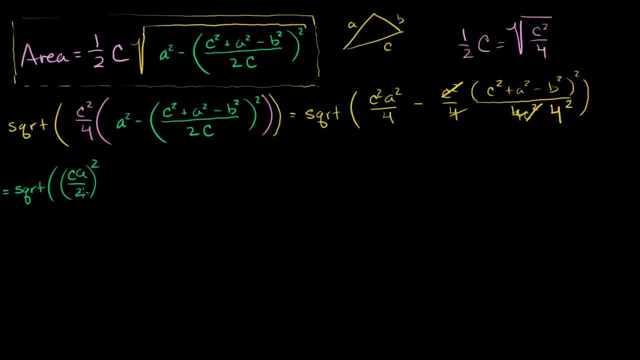 squared squared. If I square it, that's the c squared, a squared over 2 squared over 4.. Minus- I'm going to write this whole thing as an expression- squared. so that's c squared plus a squared minus b squared. 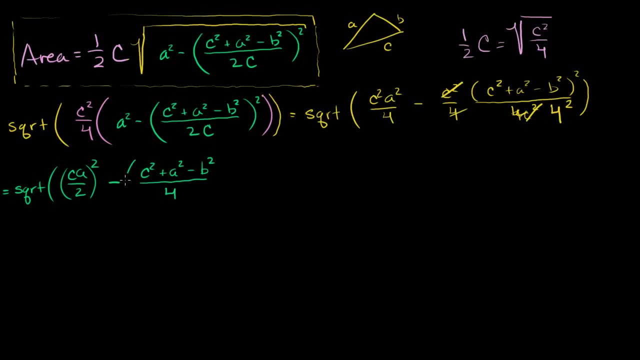 over 4.. And we're squaring both the numerator and the denominator. We squared both the numerator and the denominator. Now this might look a little bit interesting to you. Let me make the parentheses a slightly different color. You might remember from factoring. 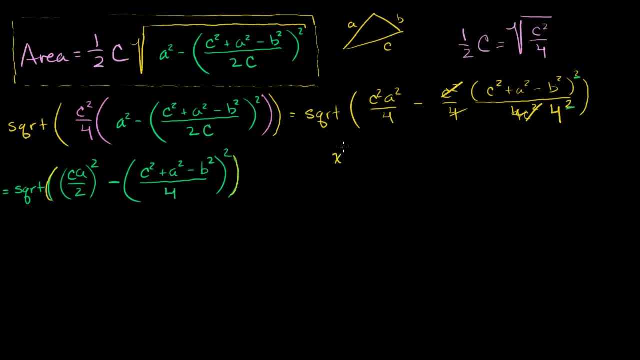 From factoring polynomials that if I have something of the form x squared minus y squared, that factors into x plus y times x minus y, And we're going to be using this over and over again. Now, if you call c a over 2 x and you call this whole big. 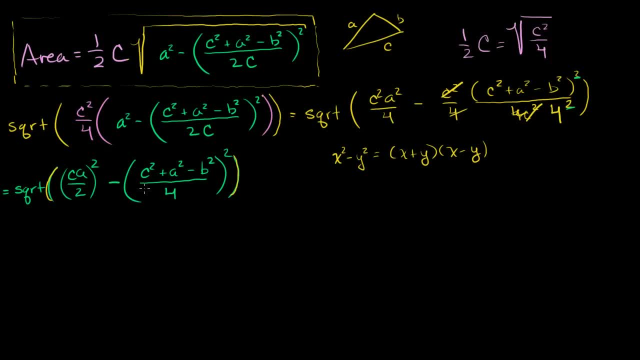 thing y. then we have x squared minus y squared. So we can factor it. So this whole thing is going to be equal to the square root of x plus y, Or in this case it's c a over 2 plus the y. 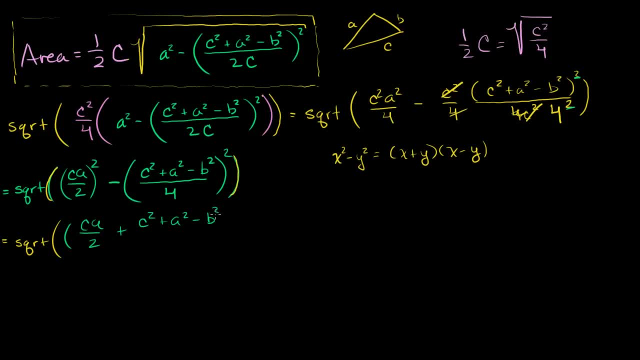 Which is c squared plus a squared minus b squared over 4.. Times x minus y. so this is our x, c, a over 2, minus all of this business over here. Or, even better, let me just say plus And then let me just write the negative. 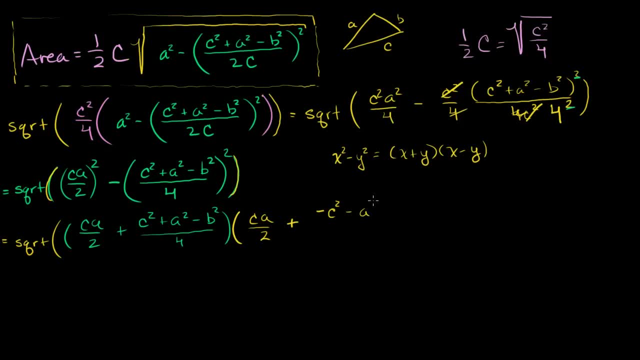 So plus minus c squared, minus c squared. And then let me just write the negative. So plus minus c squared minus a squared. So plus c squared minus a squared, minus b squared over 4.. minus a squared plus b squared, all of that over 4.. 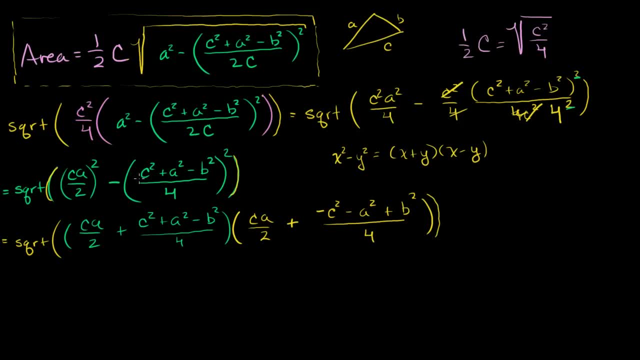 So all I did here, all I did here as I said, this is the same thing as this plus this, this plus, this times, this minus this, this minus. I just multiplied, I just said plus the negative of this. So minus c squared, minus a squared, plus b squared. 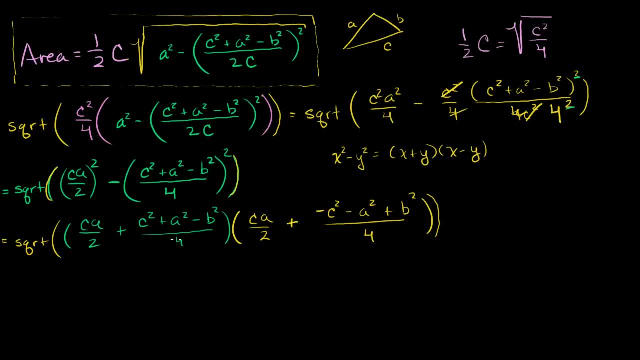 All I did is that right there. Now let's see if we could simplify this, or if we could add these fractions. Well, we can get a common denominator ca over 2, that's the same thing as 2ca over 4, just. 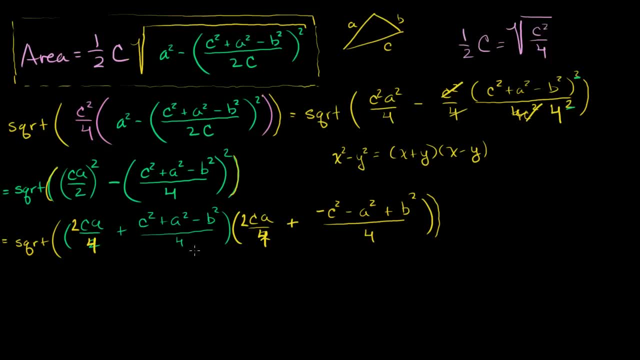 multiplying the numerator and the denominator by 2. And now we can add the numerators, So our whole expression is now going to be equal to the square root. of this first expression will become- and I'm going to write it this way: 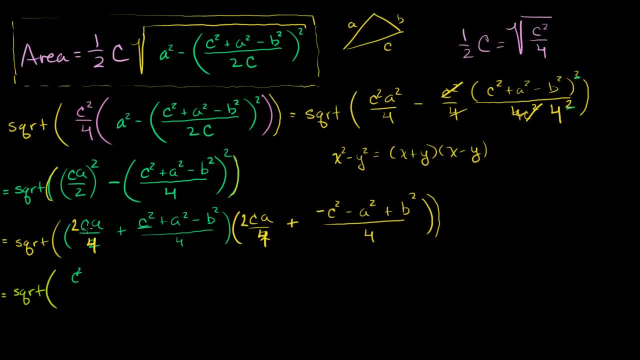 I'm going to write it this way. I'm going to write c squared plus 2ca, plus a squared minus b squared, all of that over 4.. That's our first expression, And then our second expression is going to become well. 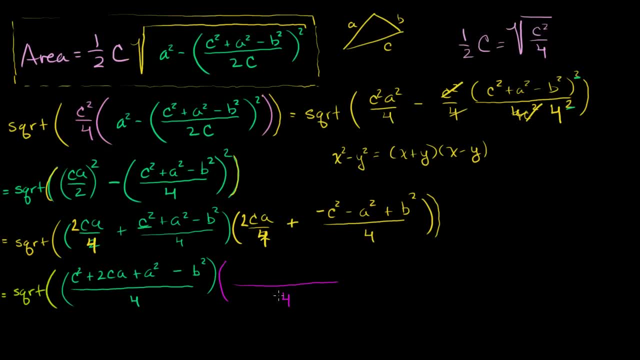 everything's going to be over 4, so I'll just write that right now: everything over 4.. So we could write this as b squared, b squared. And then we could write this as b squared minus c squared minus 2ca plus a squared. 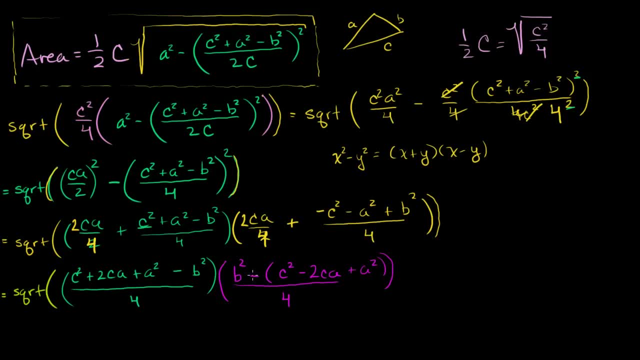 Let's make sure. I have a minus a squared here. plus times a minus, still it's a minus a squared. I have a plus 2ca over here. minus times a minus, that's plus 2ca. I have a minus c squared here. I have a minus c squared here. 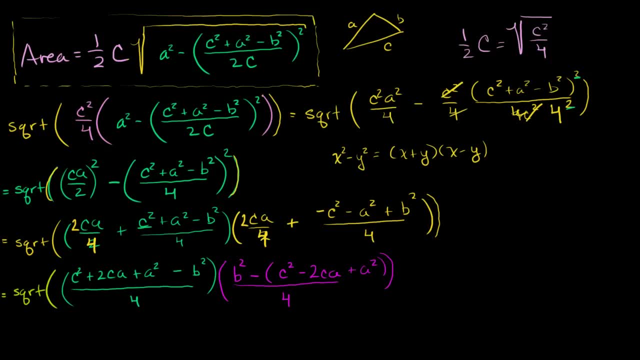 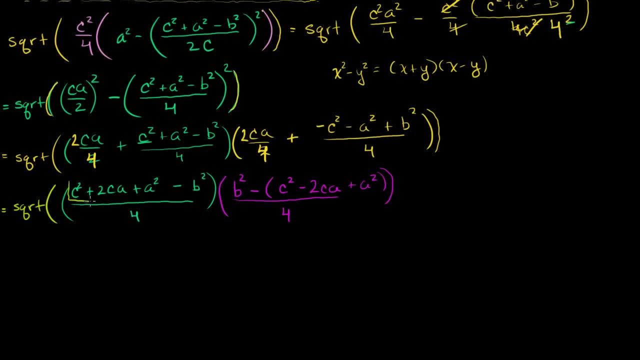 So these two things are equivalent. Now, the next thing we need to recognize, or hopefully we can recognize, is that this- over here this might get a little bit messy- that's the same thing as c plus a squared. Let me write this: 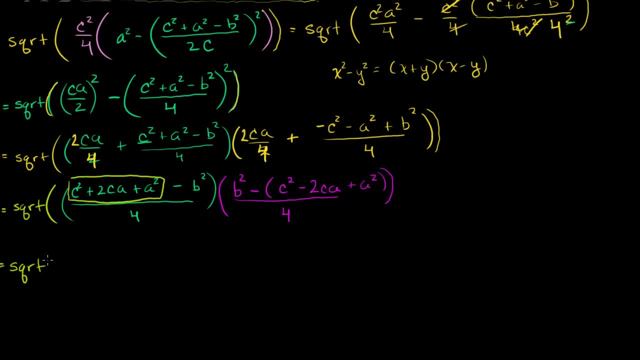 This is equal to the square root. open parentheses of this over here is c plus a squared. So this over here is c plus a squared minus b squared over 4.. That's that first term And then the second term. this over here is the same thing as: 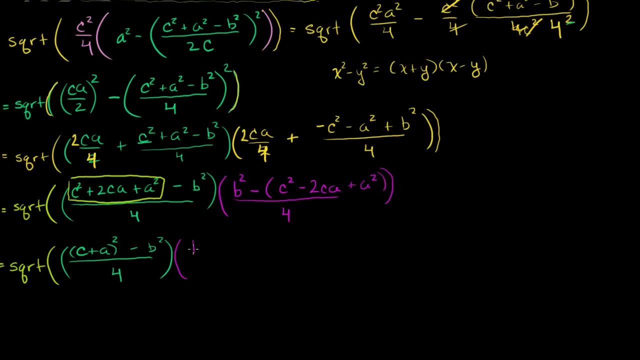 c minus a squared. So that whole thing will simplify to: b squared minus c minus a squared, All of that over 4.. So we're making some headway. As I told you, this is a hairy problem, but we're seeing some. 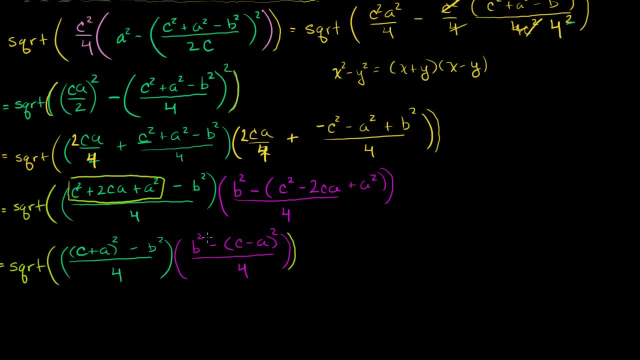 neat applications of factors. We're factoring polynomials and we're seeing how a fairly bizarre looking equation can be transformed into a simpler one. Now we can use this exact same property. We have that pattern: Something squared minus something else squared. 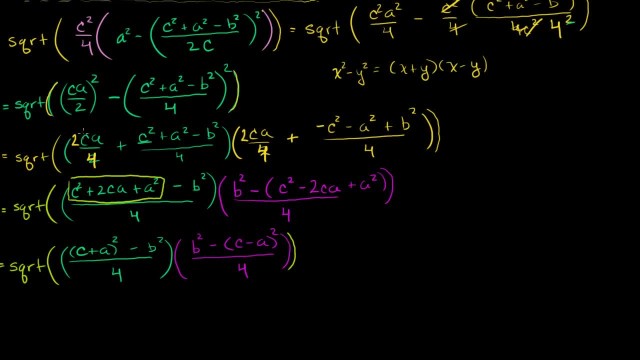 Something squared minus something else squared, So we can factor it out and I'll do it in the same line. So this is going to be equal to. I'm going to write a little bit small, just so I don't run out of space. 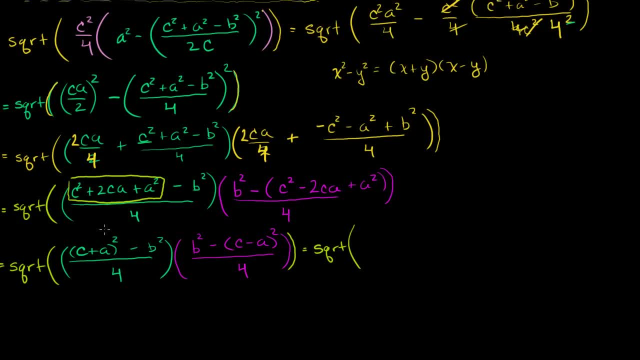 The square root. this will factor into this plus this. So c plus a plus b Plus b, Times c plus a minus b. right, It's this exact same pattern that I did over here. This is x squared. this is y squared. 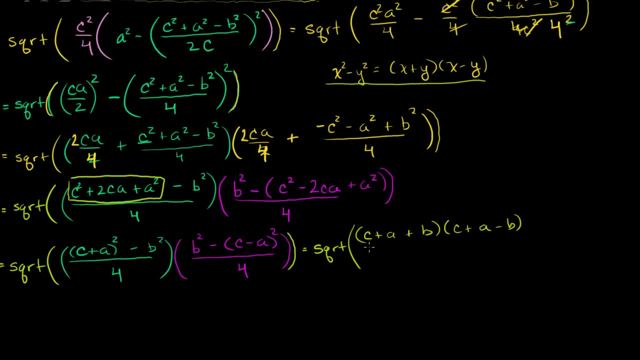 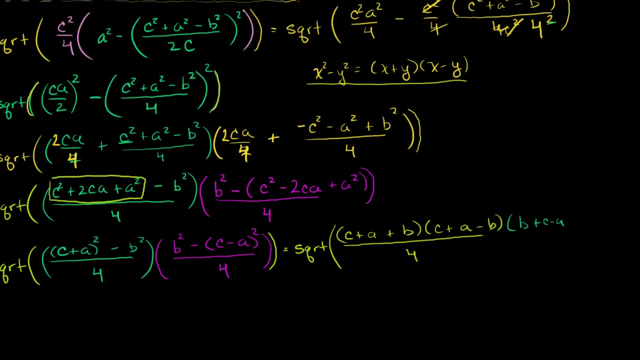 So times c plus a minus b, All of that over 4.. And then we have this one. This is going to be b plus c minus a. So we're going to have b plus c minus a. Let me scroll down to the right a little bit. 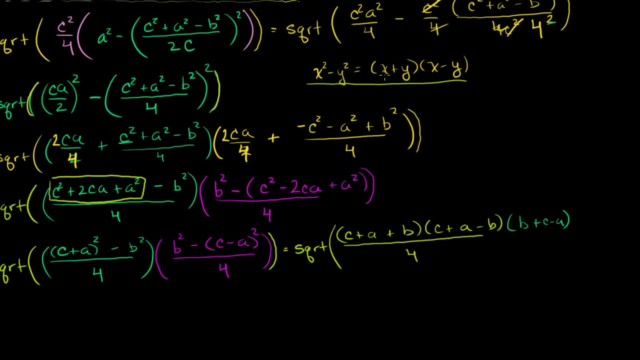 Times: b plus c minus a right. That's x plus y Times. b minus c minus a, Or that's the same thing as b minus c plus a. That's the same thing as b minus. this is the same thing as b minus c minus a right. 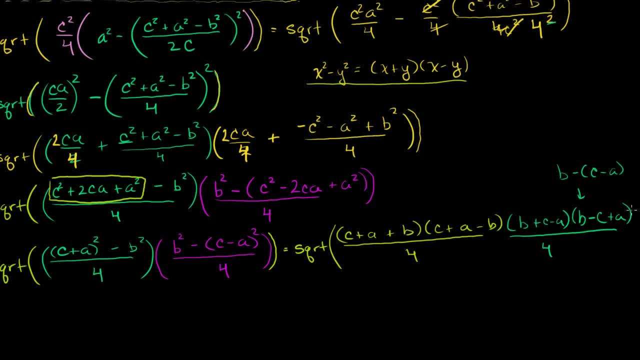 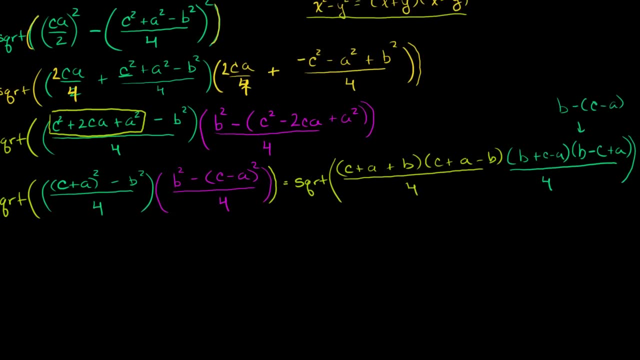 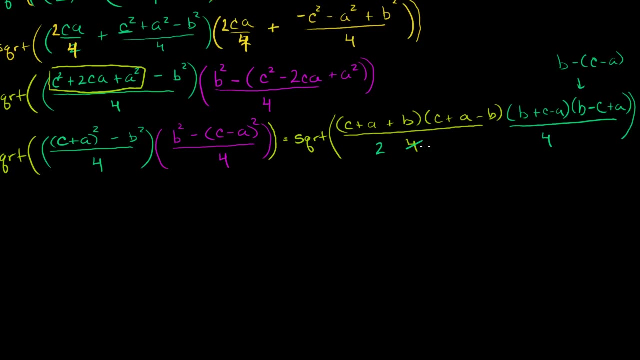 All right, and all of that over 4.. Now I can rewrite this whole expression. I don't want to run out of space. I can rewrite this whole expression as I could write. well, 4 is the product of 2 times 2.. 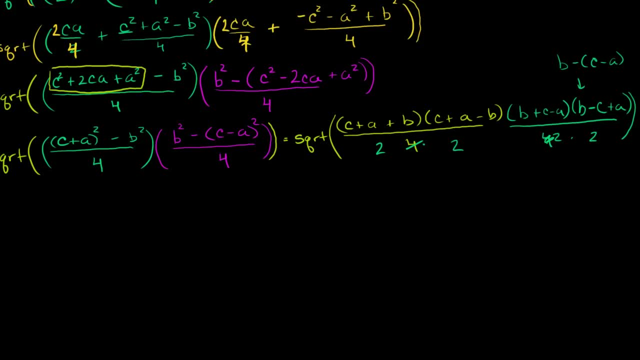 4 is the product of 2 times 2.. So our whole area expression has been arguably simplified to. it equals the square root, And this is really the home stretch of this right here, which I could just write as a plus b plus c. 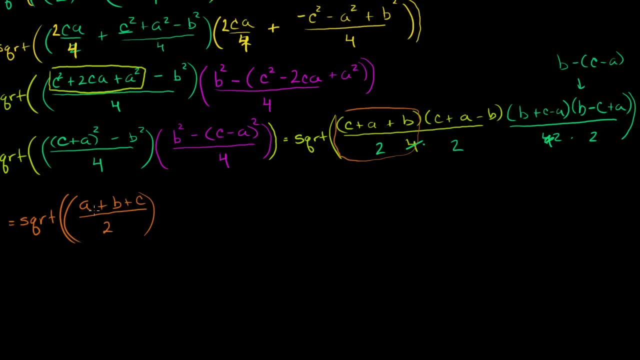 Over 2.. That's that term, right there. Times this term Times that term. And let me write a simplification here: c plus a minus b, That's the same thing as a plus b plus c minus 2b. These two things are equivalent, right. 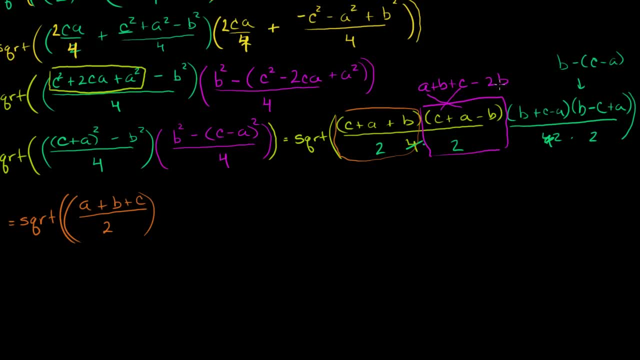 You have an a, you have a c, and then b minus 2b is going to be equal to minus b. right b minus 2b, That's minus b. So this is going to be this. next term is going to be a. 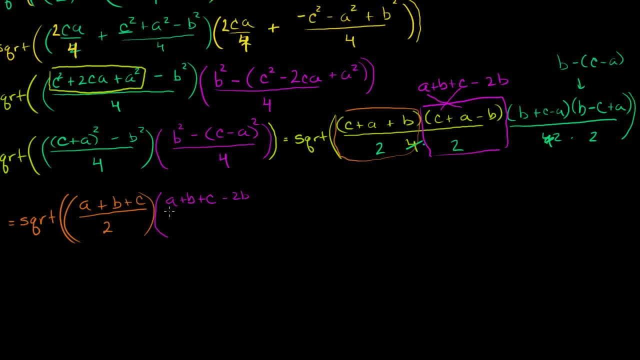 plus b plus c minus 2b over 2.. Or instead of writing it like that, let me write this over 2 minus this over 2.. And then our next term right here: same exact logic. That's the same thing as a plus b plus c minus 2a. 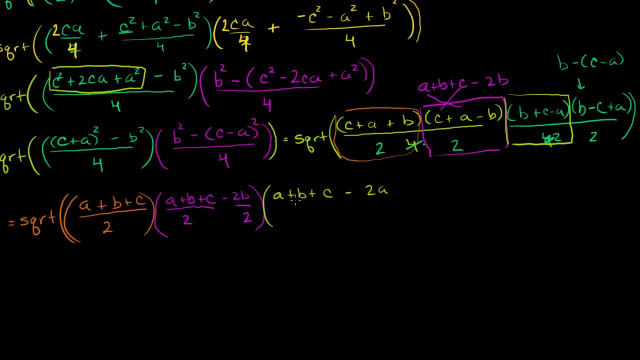 Minus 2a. All of that over 2,. right, If we add the minus 2a to the a, we get minus a. So we get b plus c minus a. These are identical things. So all of this over 2, or we can split the denominators. 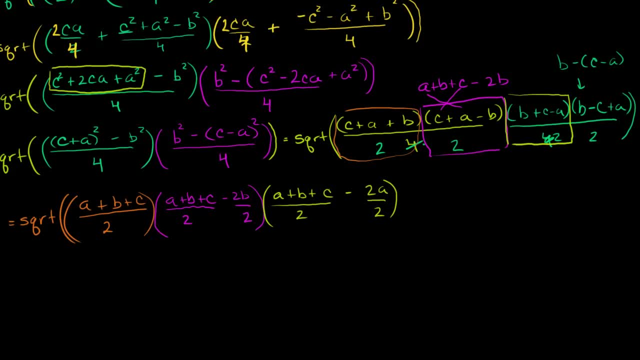 just like that, over 2.. And then one last term, and you might already recognize the rule of Heron's formula popping up. I was thinking not the rule of Heron, Heron's formula, That term, right there is the exact same thing as a plus 2a. 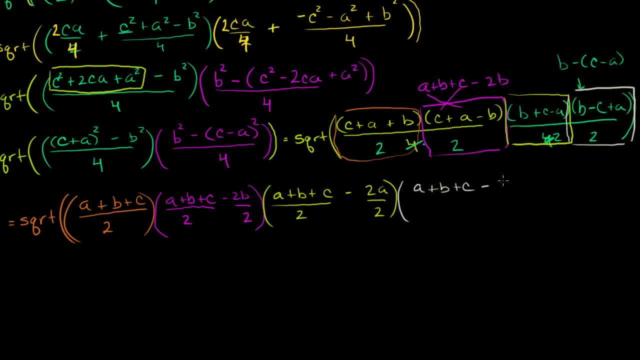 That's the same thing as a plus 2a. That's the same thing as a plus b plus c minus 2c. right, You take 2c away from the c, you get a minus c, and then you still have the a and the b. 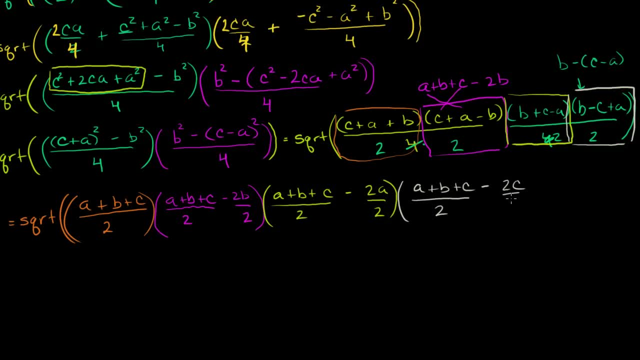 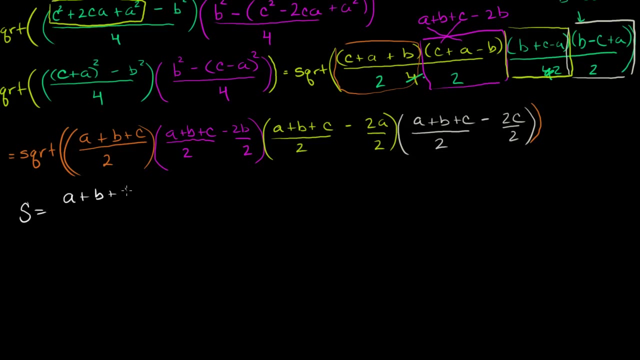 And then all of that over 2.. Write that over 2 minus that over 2.. And of course we're taking the square root of all of this stuff. Now, if we define an s to be equal to a plus b plus c over, 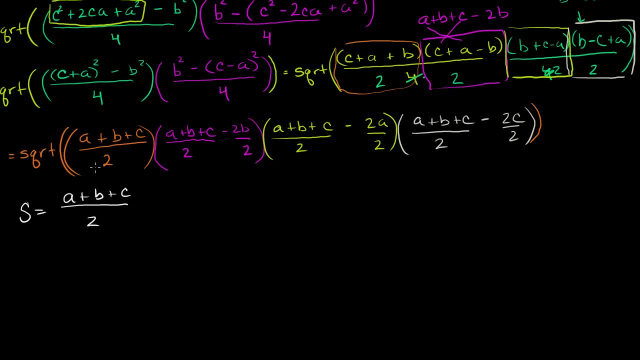 2.. Then this equation simplifies a good bit. This right here is s. That right there is s. That right there is s. That right there is s. And these simplify a good bit too. Minus 2b over 2, that's the same thing as minus b. 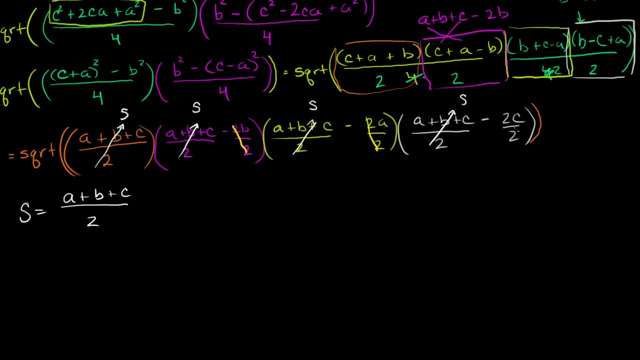 Minus 2a over 2, that's the same thing as minus a. Minus 2c over 2, that's the same thing as minus c. So this whole equation for our area now becomes: our area is now equal to. 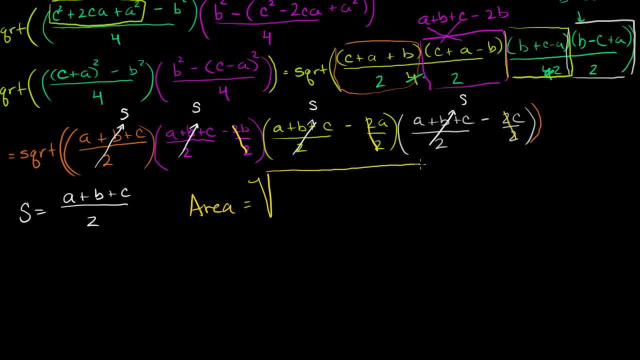 I'll rewrite the square root, The radical, the square root of s. That's that, right there, of s Times. I'll do it in the same colors: Times s minus b Times s minus b Times. this is s minus a. 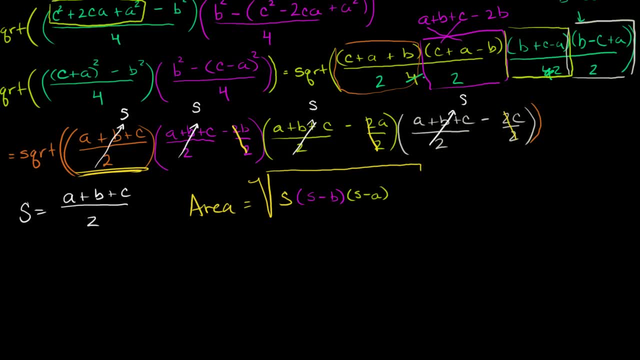 s minus a Times and we're at the last one. s minus c, s minus c, And we have. We have proved Heron's formula. It's the exact same thing as what we proved at the end of the last video. 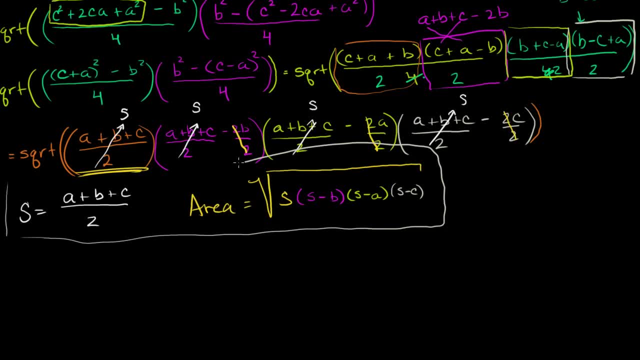 So this was pretty neat, And we just had to do a little bit of hairy algebra to actually prove it.